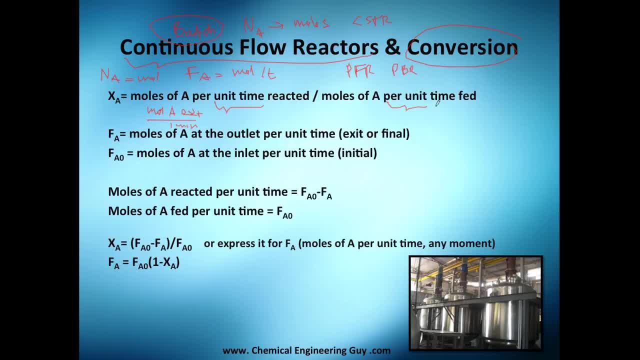 Per the amount of moles of A per unit time that you're being fed or you are feeding. So the moles of A that you fed for those minutes or that minute, Okay, So yeah, Once again, let's establish F of A or flux or flow of A, its moles of A at outlet per unit. 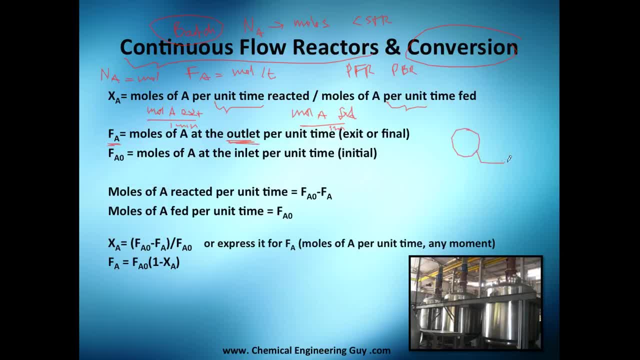 time or at the ending. So if I got this reactor, let's say F of A will be this number here. Now F of A0 is the moles of A per unit time Q. How is that per unit time that I transfer that there's difference. 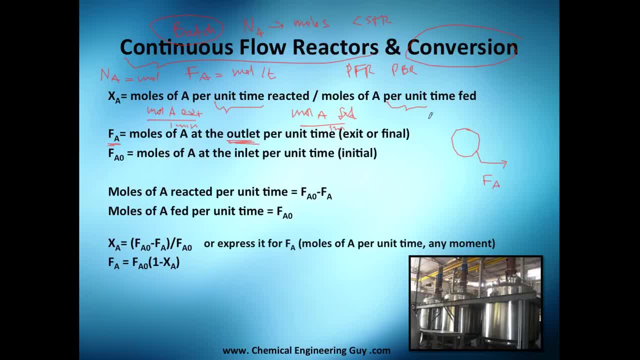 ¿A was the most joule, D, Q, No, that's my mistake from the previous chapter. the moles of A at the inlet per unit time. so let's say this is F of A zero or initial, which is mole of A per unit time. this is also same mole of A per unit time. okay, now I need. 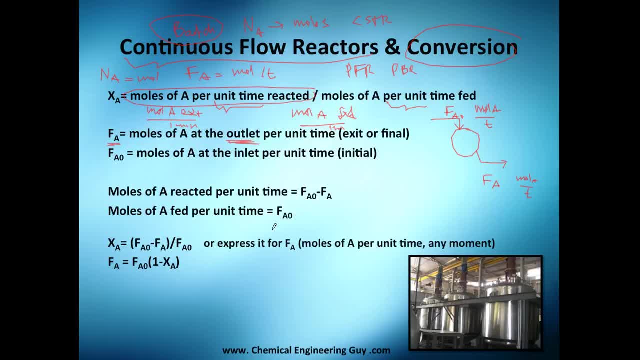 to get this quantity? how do I get the moles of A being reacted per unit time? that's very easy. similar to the batch reactor, is the moles and feeding initially, which is this flow minus the moles that are going out, the moles that are not reacting. so, of course, if I have 100, 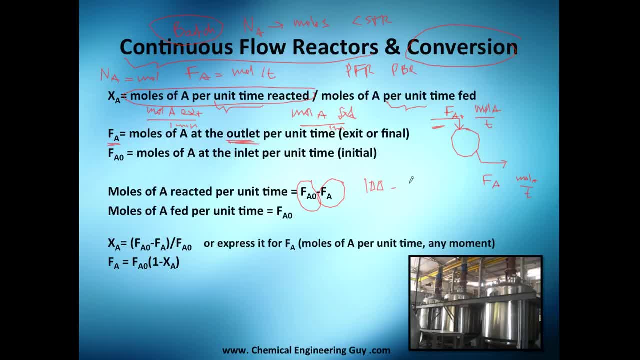 moles being fed per minute, and I'm taking out 20 moles per minute. I have a difference of 80, and what does that mean, though? that 80 means they are disappearing or they are converging, and I have a difference of 80, and what does that mean, though? that 80 means they are. 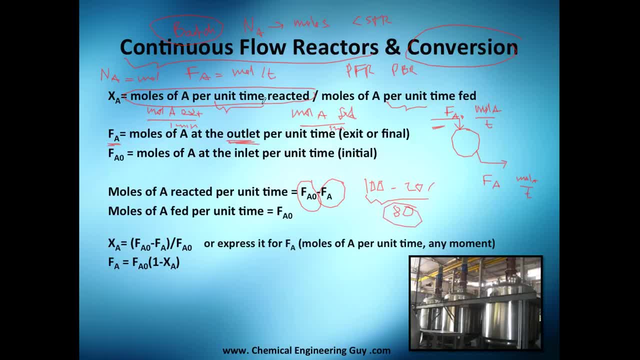 converting to products. so that is the value I want to put in this equation now, moles of A fed per unit. time it's easy. they actually tell you it's F of A zero. so once again we go to the definition of conversion and we show that this divided by this is my conversion, or once. 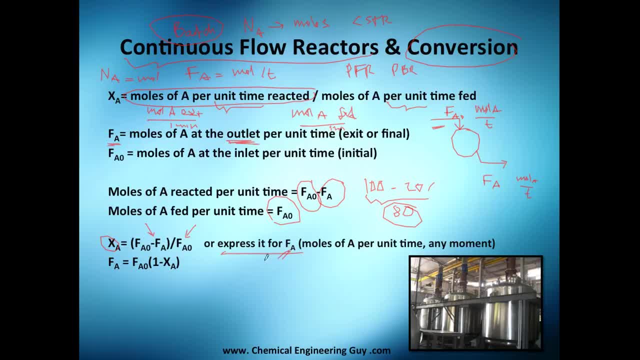 again, as you saw in my batch reactor, it's way better to use it as a function of a F of A. you know you have this here. this will be a constant, probably. they will tell you always and the conversion is also normally: choose you, choose a conversion or you. 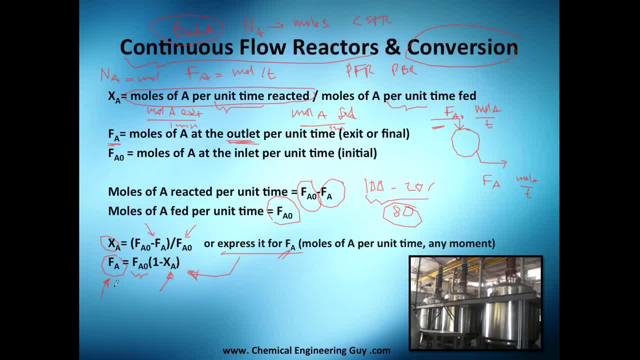 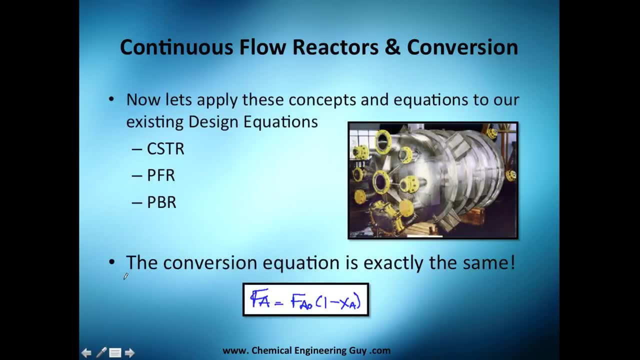 set a conversion and then you see how much flow you will get. so, yeah, like we got this once, we got this. actually, this equation is what they wanted. sorry for forgetting the video, but it's very important to get the idea of this. now let's apply these concepts. 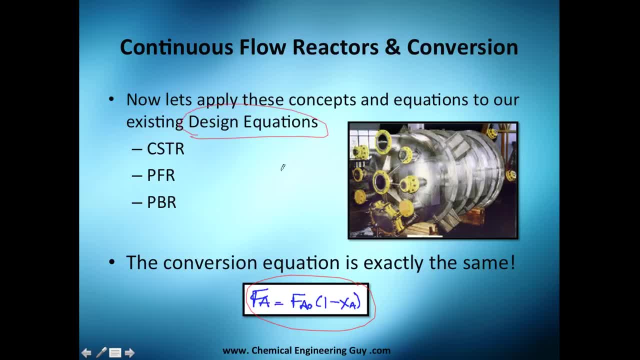 and equations to our existing design equations. hopefully you know what I'm talking about and hopefully you know what those letters mean, because if you don't know what's that, please go back on the playlist, because you really need to know in order to continue. so, yeah, we're going to use this equation. 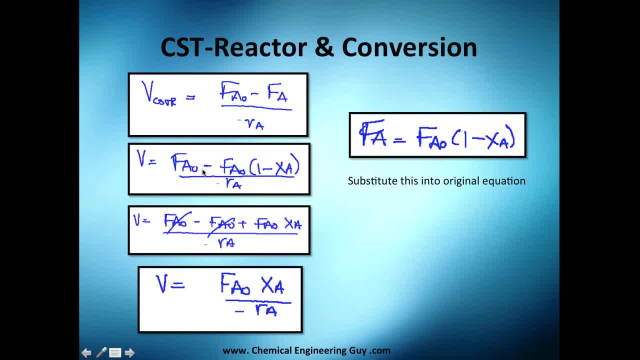 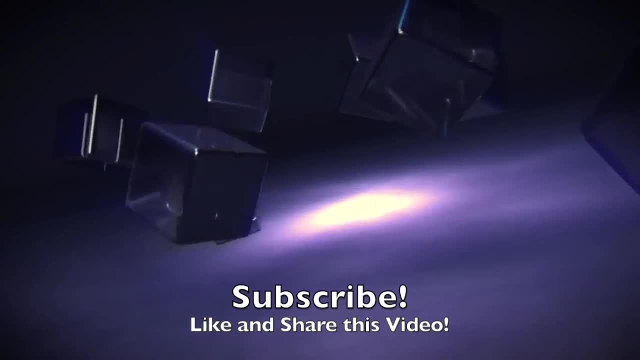 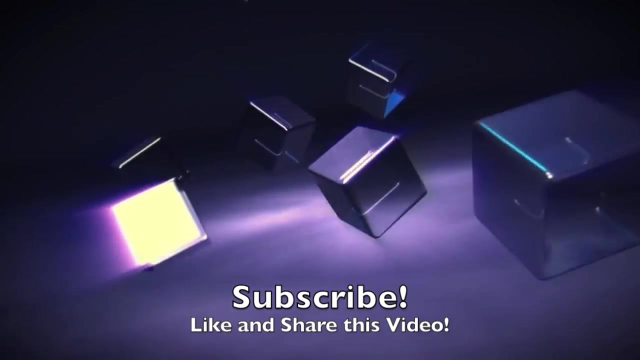 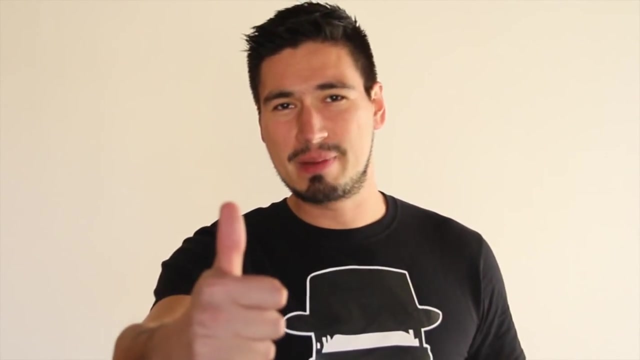 for every continuous flow reactor. in the next video we're going to see the continuous tier tank reactor and, yeah, essentially just to substitute this formula. but yeah, better tell you that in the next video. um, what's up guys, it's me chemical engineering guy. so if you like that video, why not push the like button? 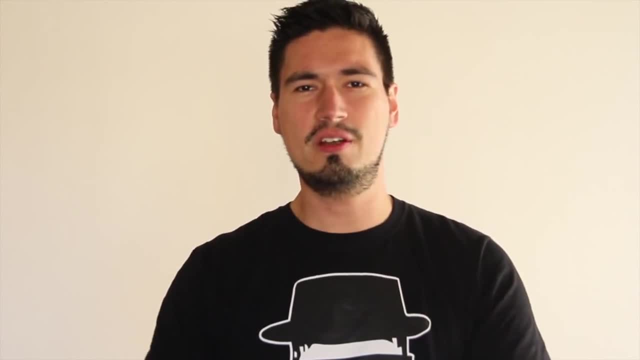 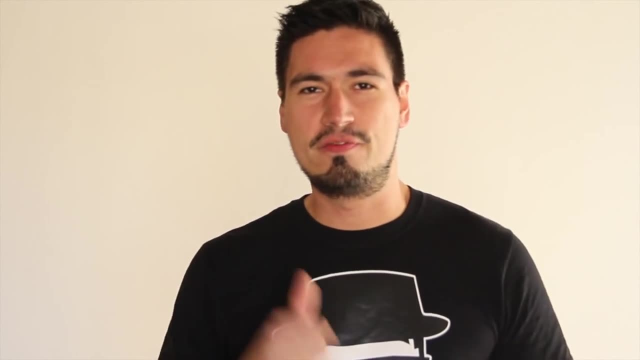 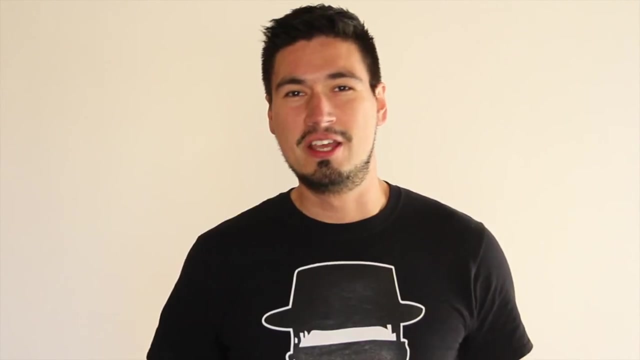 to know if you're liking the videos or if I should be changing something or I should be adding something. taking out content, whatever. Also, sharing is caring, so if you've got any kind of friends, teachers, colleagues or whatever kind of person that might be interested in this type of content, why not share it? 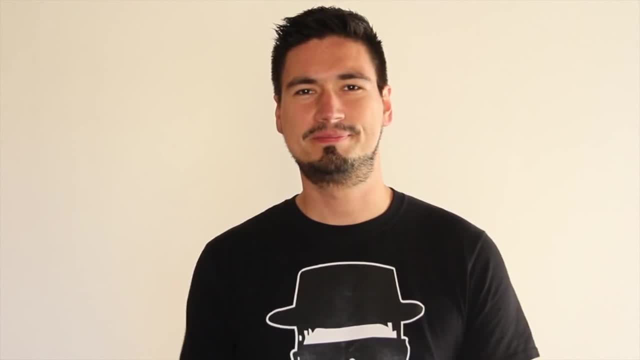 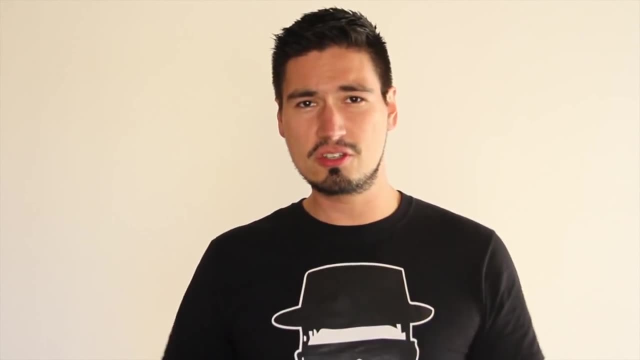 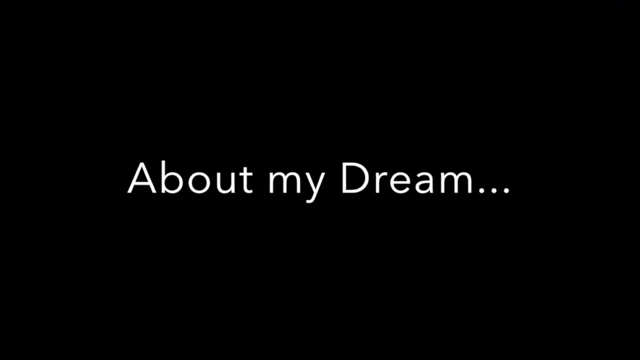 Sharing helps our community to grow faster- in members and in content. If you want to keep track of my activity- videos, uploads, experiments, playlists, whatever content I'm getting on YouTube- be sure to click the subscribe button. Subscribing to the channel is totally free, guys. 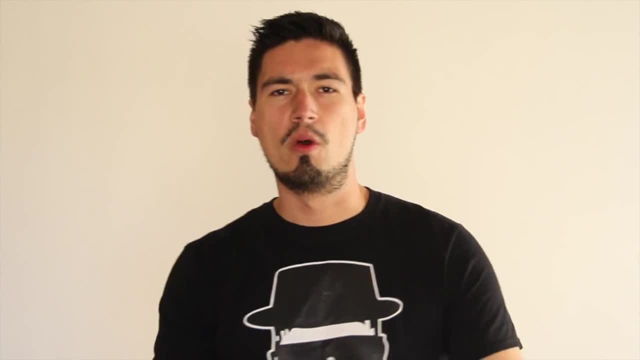 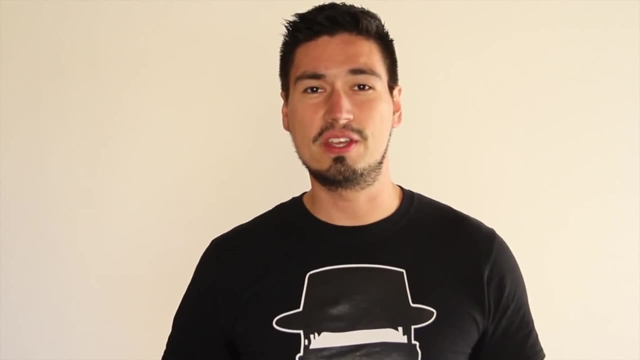 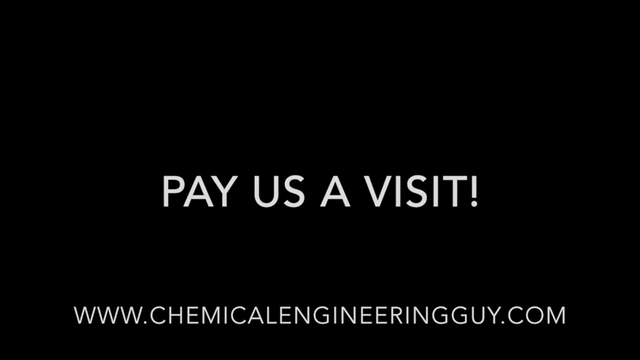 My dream is to create an online academy of chemical engineering where everyone can access it in the world. Imagine a place in which the student, the teacher and the engineer get the best of each other. Thank you very much, Thank you, thank you. thank you, guys, for the support and the love.